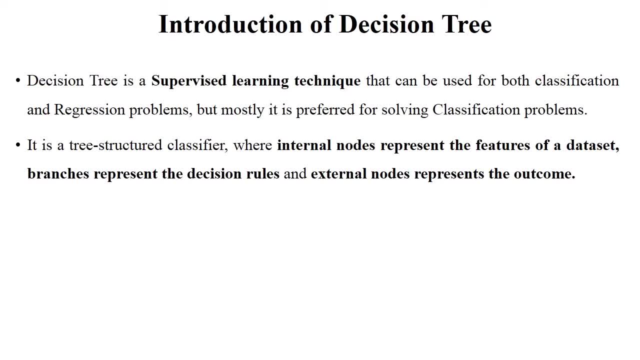 Okay, so first topic is introduction of decision tree. I think you all are familiar with the concept of tree Here in machine learning. decision tree algorithm is included in supervised learning technique. Decision tree algorithm generally used for classification as well as in regression problem, But most preferably that will be used for solving the classification problem. Decision tree represent a data set, in particular hierarchical format. There are internal nodes and 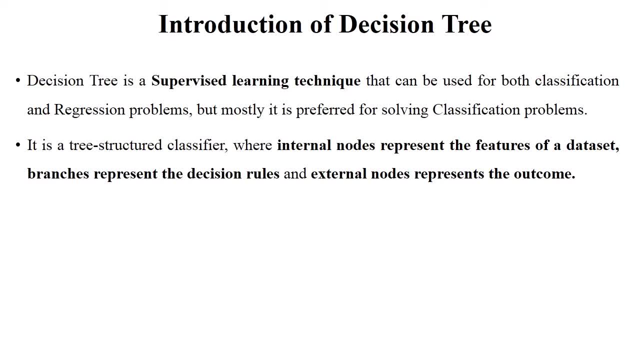 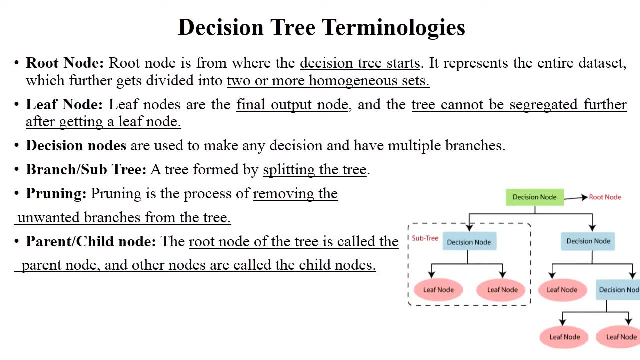 external nodes, Okay, and internal nodes represent the features of data set and external node represents the outcome. So let's see with terminologies. Okay, now see here in this diagram, These are the same decision tree terminologies. The first node is called as root node, That is, your main decision node, or parent node. So root node is from where the decision tree start. The next left subtree and right subtree is there, Okay, and all the decision nodes. 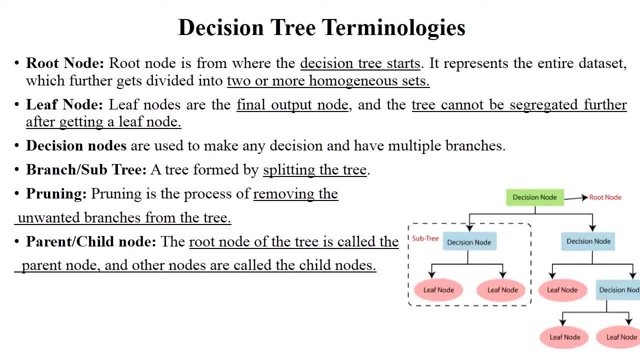 are called as internal nodes. These decision nodes are used to make the particular decision and particular conditions are stored there. Okay, as per the condition you need to decision tree classify the data. and last node are called as external nodes. This external nodes also called as leaf node, So leaf node stored the final output of that particular condition into the particular node. So parent node, internal node, are called as decision node. 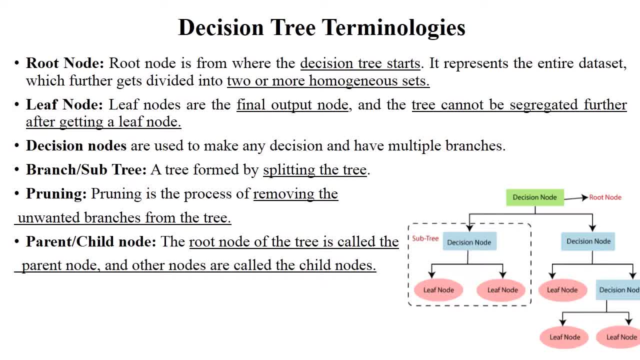 And external node are called as leaf node. So there are various sub trees: left subtree and right subtree. The next concept is pruning. Pruning is a process of removing the unwanted branches from the tree. means the data set that will be required for only the particular decision and particular condition. Only those data are represented into the hierarchical format. So these are the terminologies in decision tree. I will explain with example. So before start the decision tree, there are some concepts and 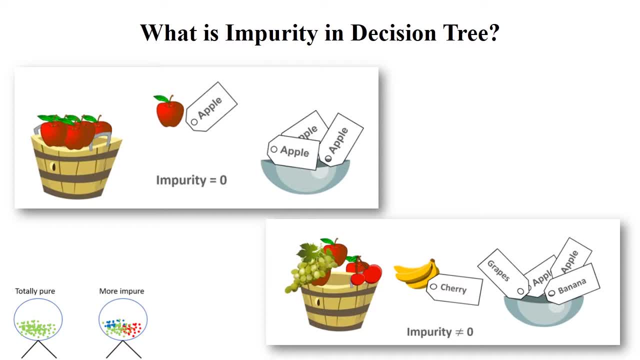 there are some methodologies in decision tree. So let's see. the first concept is impurity. So what is impurity in decision tree? See, in the first diagram. In this first diagram there are data set of images are given and also labels are given. In this data set there are Apple images are there and labels. Apple is given. So there are multiple apples are there and there are Apple labels are there, right, So this Apple image is matched with the Apple label. 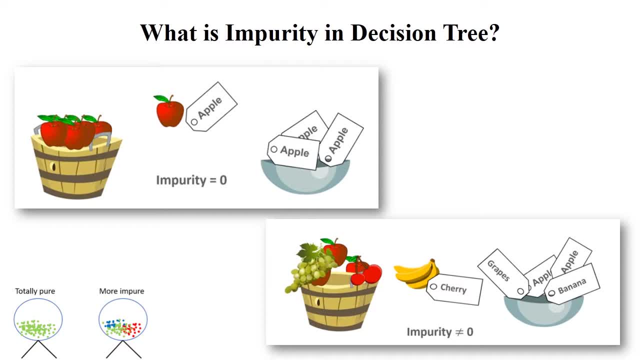 So probability is 100% because there are only Apple images. is there, right? Means their impurity is equal to zero. The 100% match. now see here in this below diagram: There are multiple fruits. are there? There are grapes, apple, bananas and there are various labels. are there as per the fruits, right? But the probability is not 100% to. the particular fruit is matched with the particular label. So at that time there are, impurity is not equal to zero. 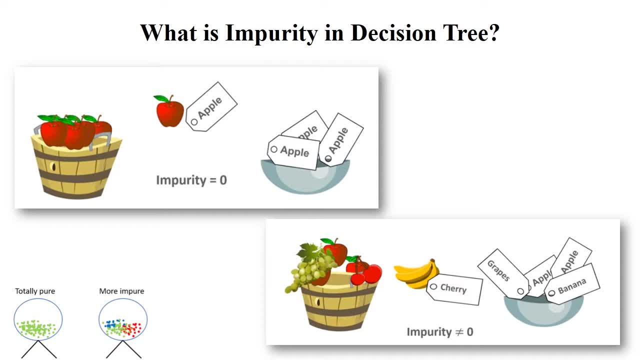 0. so this is a concept of impurity. when there there are probabilities hundred percent to match the particular data set with particular level, so impurity is 0. and when there are probabilities not a hundred percent, at that time impurity is not equal to 0. so this is a concept of impurity. 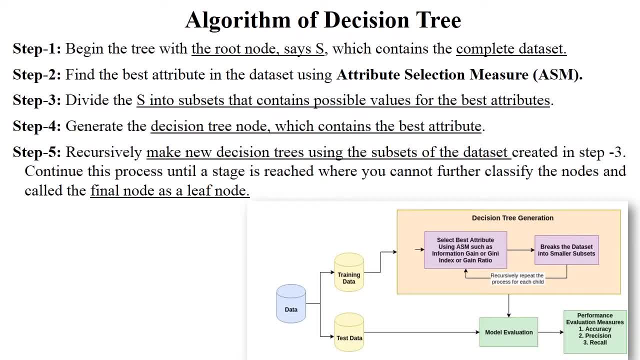 in decision tree. now this is the algorithm of decision tree, so i will this, i will explain this algorithm step by step with the some terminologies or attribute selection major in decision tree. so basically, in algorithm you need to start with the root node, after that you need to calculate. 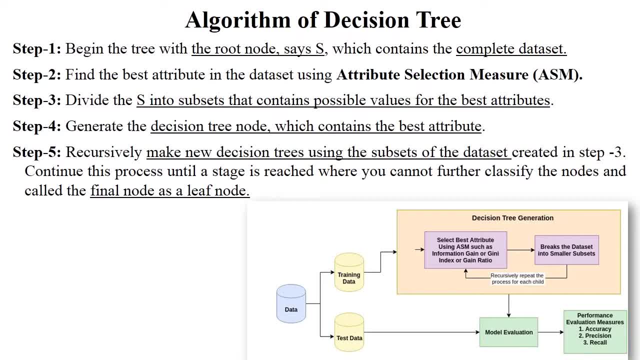 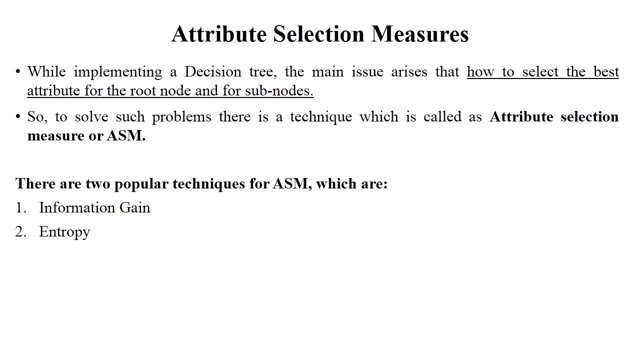 attribute selection majors. i will explain this. or next, you need to calculate possible values, that decision tree node and best attribute and after that final nodes as a leaf node represent the outcomes. so this is the algorithm of decision tree. okay, so in algorithm of decision tree, the one 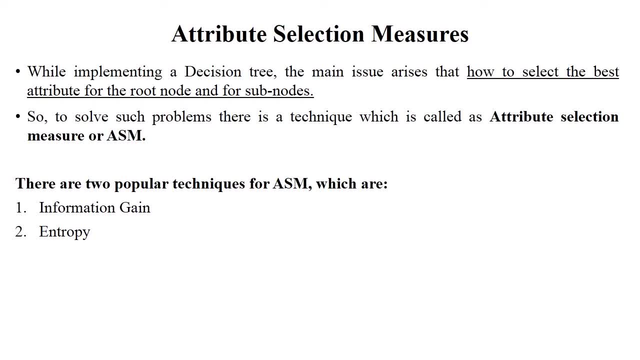 of the most important concept is attribute selection major, which is also called as impurity. so this is a concept of impurity in decision tree, so this is a concept of impurity. ASM- so attribute selection measure, generally used to represent how to select the best attribute for the root node and for the sub node, because in each and every node you need to take a. 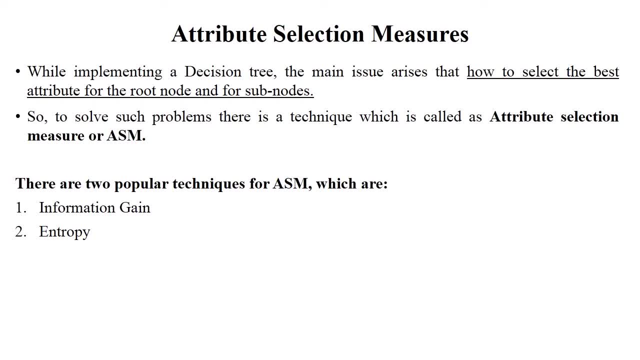 decision: either yes, then it move forward to the left subtree, if it not no, then it move forward to the right subtree. right, so it completely depend on attribute selection measure. so in attribute selection measure there are two popular technique. one is information gain and another is entropy. so let's see, okay. so first we will learn about entropy. what 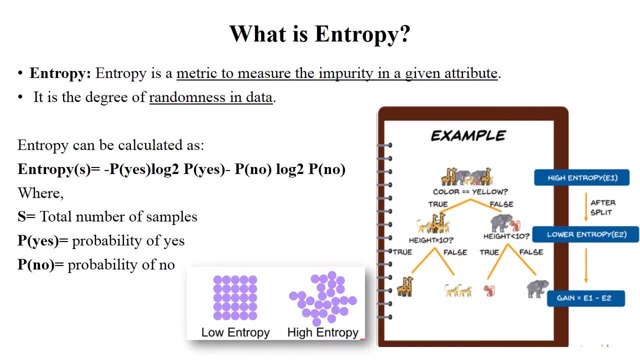 is entropy. so, simply, entropy means degree of randomness in data, means how randomly data is present at the time that entropy is high. let's see, let's learn with the example. see here in this given example, the first as a root node: there are lot of animals are present. 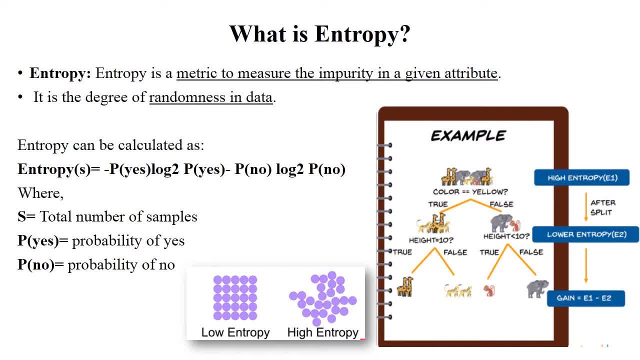 there, right, there are a giraffe, then elephant and other animals are present. there are animals are present means there are random data is there at that time. their entropy is high. when you split this data, set as per the particular condition, for example, color equal to yellow, this is our condition. and when you split this data as per the condition at that time- yellow. 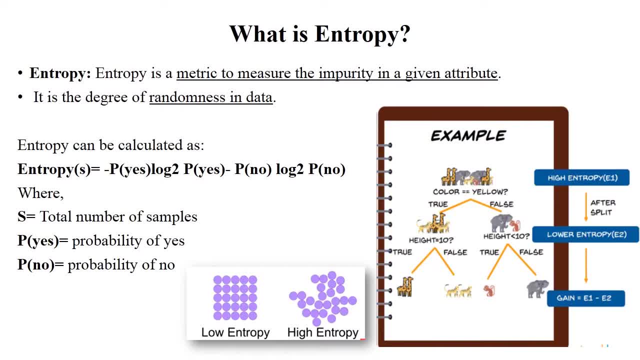 color animals are present into the one side and other than yellow color animals are present into the another side. that is true or false. so at that time- see here there is a randomness- is decreases. so at that time there is a lower entropy as compared to root node. again there, 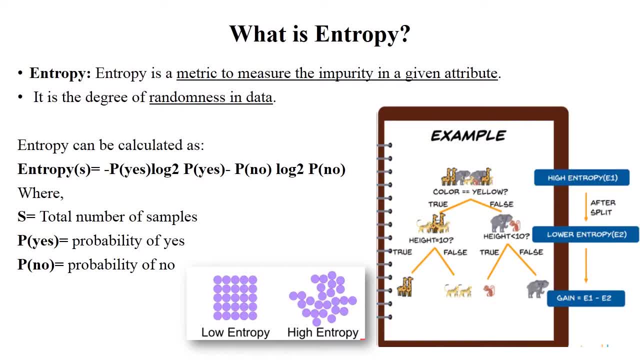 are some particular condition, that is suppose height equal to 10, this animals are stored into the left subtree. and height is greater than equal to 10, this animals are stored into the right subtree. in this way, so again, this particular data set will be sort out right. 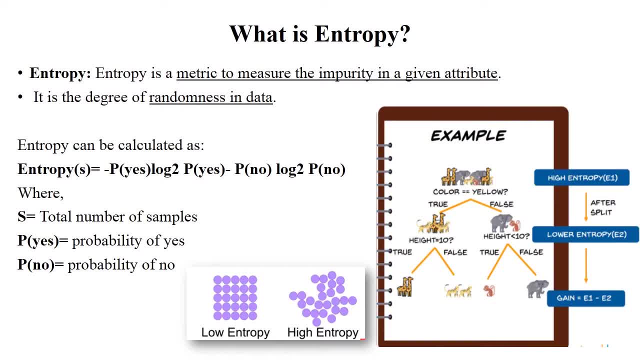 means there is a randomness of data is decreases. so at that time at the left node, entropy is lower and entropy is lower is a best way to find out the particular outcomes and particular decision. so this is a concept of entropy and if randomness of data is more so, entropy is. 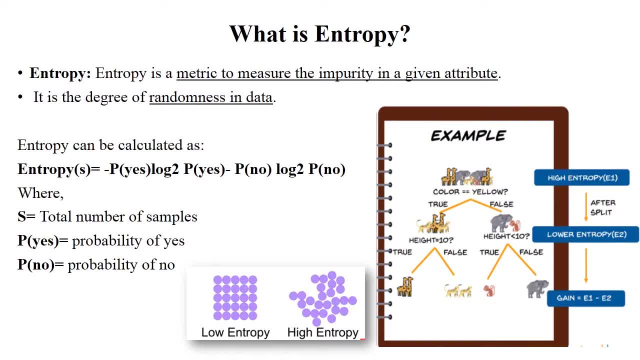 high. if randomness of data is lower, at that time entropy is low. so entropy is metric to measure impurity in given attribute. ok, so, while implementation entropy formula is this: that is, probability of yes- log2. probability of yes minus log2. probability of yes- log2. probability of no- log 2. probability of no. there will be a id3 algorithm. we will learn this id3. 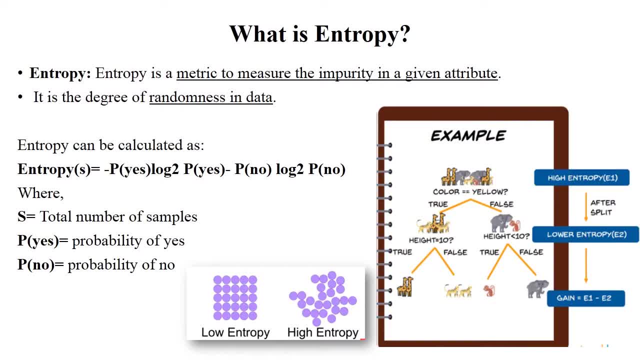 algorithm in next session. this is a decision tree algorithm, so at that time we will use this formula for calculating the entropy. here s means total number of samples, and probability of yes means how many yes and how many true values are there, and probability of no means how many false values. 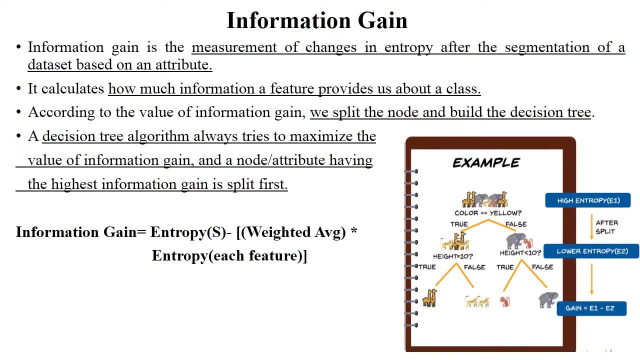 are there. so this is a concept of entropy. now the next concept is information gain. so information gain is a the measurement of changes in entropy. see here in this diagram, each and every stage entropy value is changed right. so this, as per the given condition, the data will be sought out. 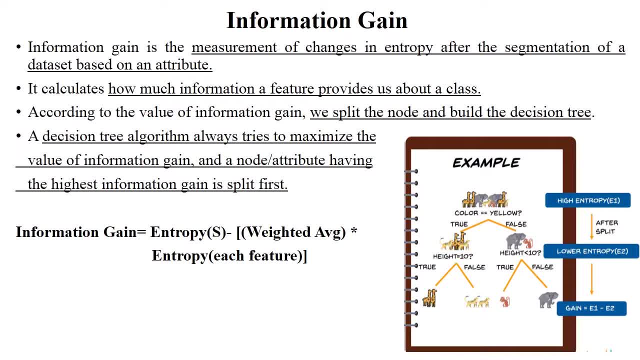 so this is again. this also called as information gain means each and every stage you need to collect the information and split the data. for example, curl equal to yellow, then split the data as per the condition, then height equal to 10, again split the data. so this thing are called as information gain means at the every stage it gain the information, or 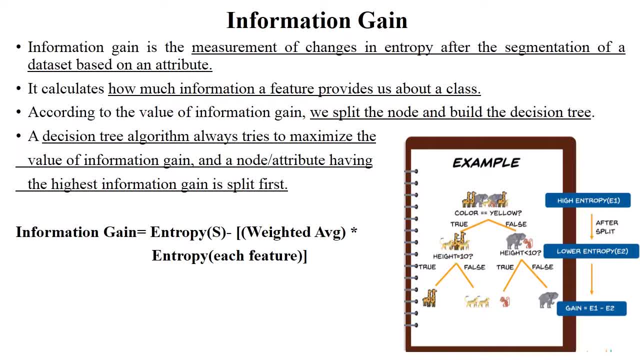 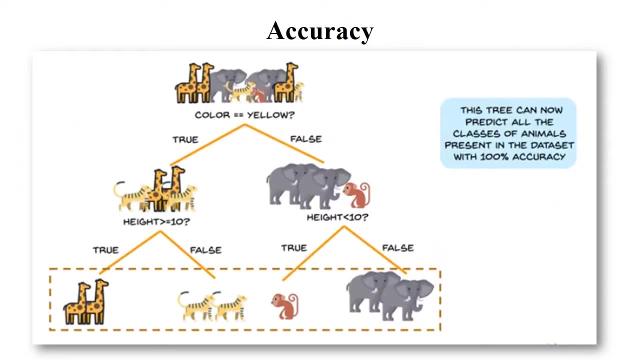 gain the particular condition. so this thing is called as information gain. so condition is proper in decision tree at that time only their accuracy is high, otherwise their accuracy is low. so the formula of information gain is entropy of s minus weighted average into entropy of each feature. so in id3 algorithm this formula is used now. next see here: this is just accuracy. 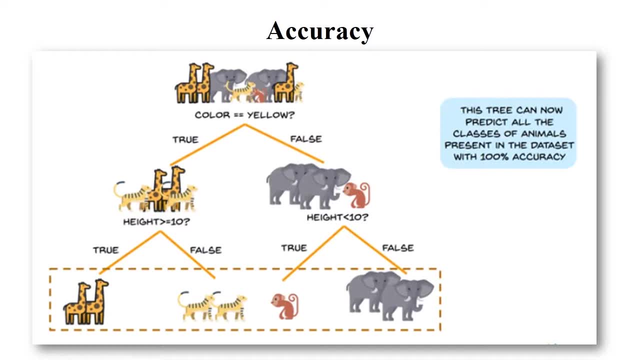 at the root node their entropy is high. so apply the condition either true or false at the time. again in this first stage or second stage, at the internal nodes their entropy is low. again, it divided into the subparts. so at the leaf node or at the end of this decision tree, their entropy is low. 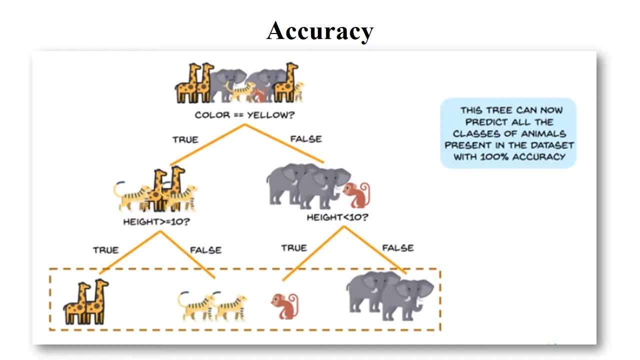 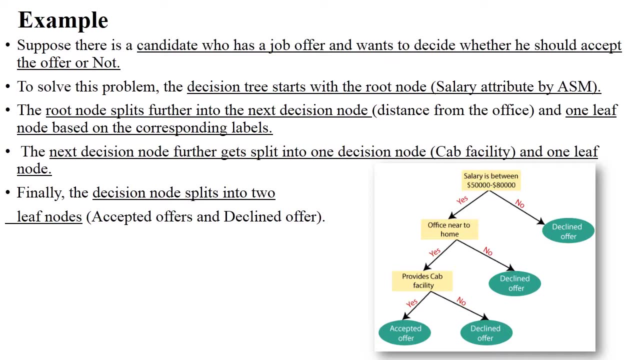 so their accuracy is hundred percent here. now let's take one example again: default decision tree. suppose the particular candidate who has a job offer letter and they want to decide whether he should accept the offer letter or not. so to solve this problem, decision tree start with the. 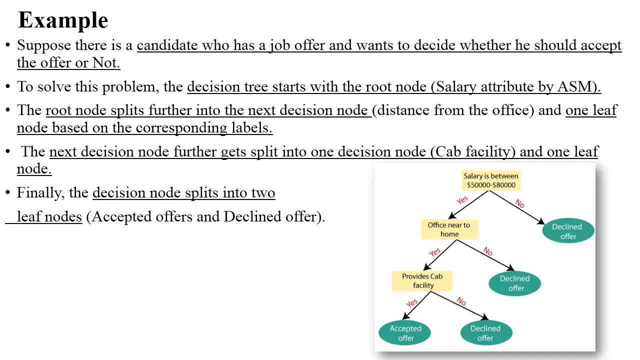 root node. see here in this diagram: salary between dollar, particular dollar fifty thousand to dollar eighty thousand. right, so the particular range is given here. so at that time they take a decision means particular office is near to home. then yes, they provide the cap facility. and yes, then they.